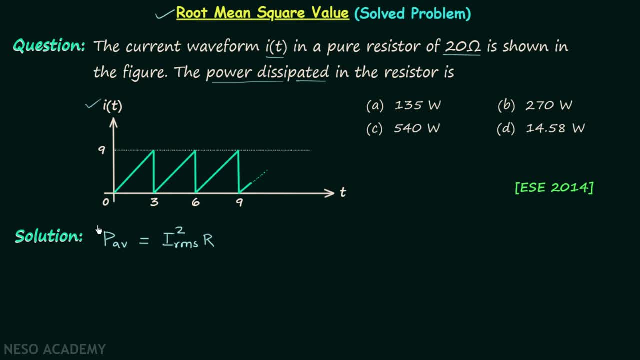 And if we can have the RMS current we can have the average power dissipated. So now we will focus on the calculation of RMS current first And we will try to have the RMS current using the waveform of I t given in the question. If you remember, in the previous lecture we found RMS current is equal. 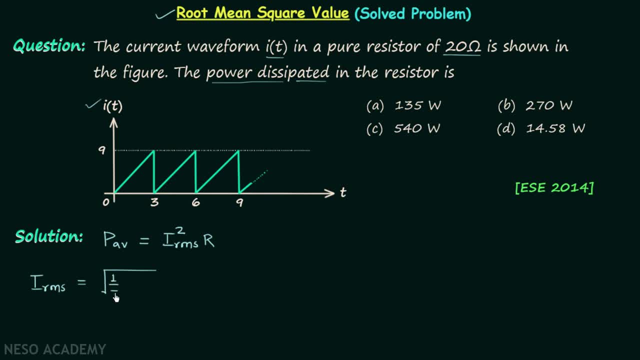 to the square root of one by t integration over one period: current I t square dt. So here we are, integrating the square of current I t over one period and then dividing it by the period And finally we are calculating the square root of I t. So the first thing we will do is to identify the period of RMS needed for I t. 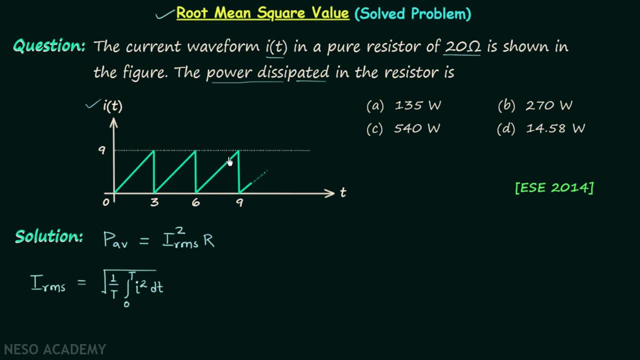 of this periodic signal. It is a periodic signal because here we have this structure, repeated infinite number of times, from minus infinity to plus infinity, And this structure is having the span from 0 to 3.. This means the period is equal to 3.. And now we will find out current. 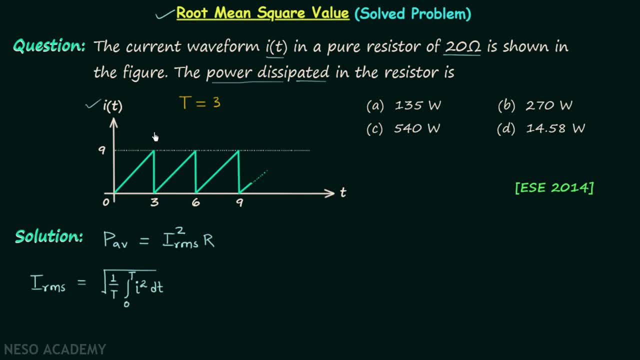 I t from 0 to 3.. And this means we will try to find out the equation of this straight line. We know the equation of straight line is y equal to mx plus c. c will be 0 because the line is passing through the origin. c will be 0.. y is equal to I t, y is I t And. 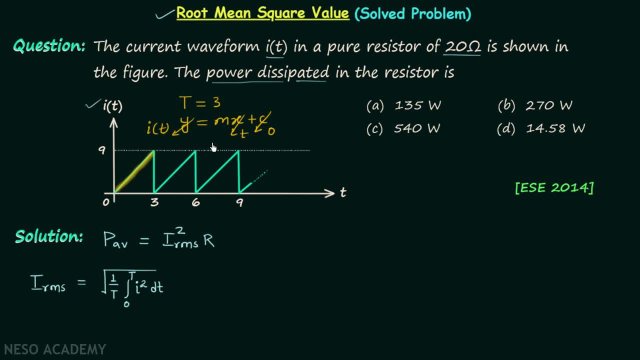 x is t. Okay, Okay, And the slope is equal to 9 divided by 3.. This means slope is equal to 3.. In this way, we have the equation of I? t. We will have I t equal to 3 t. I t is equal to 3 t from. 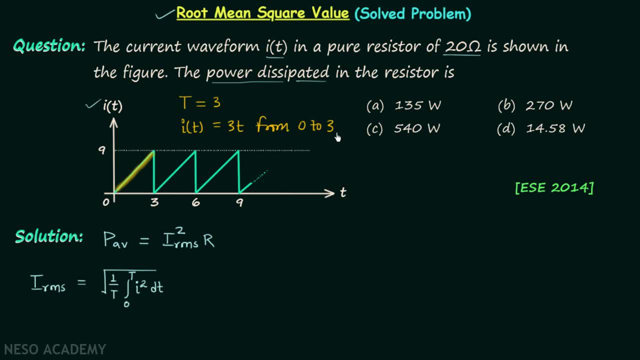 0 to 3.. So we can say that the RMS, current I RMS, is equal to under root, 1 over 3.. Period is equal to 3.. Integration from 0 to 3 square of 3 t dt 3 t square will.